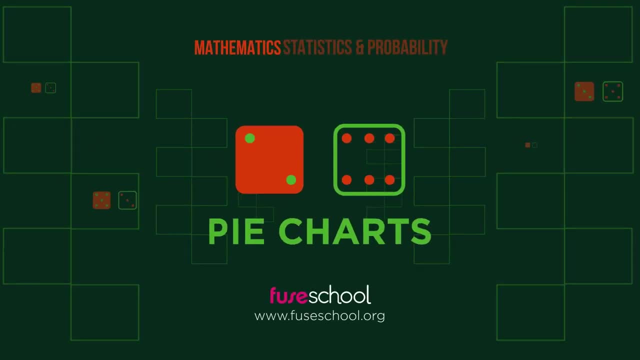 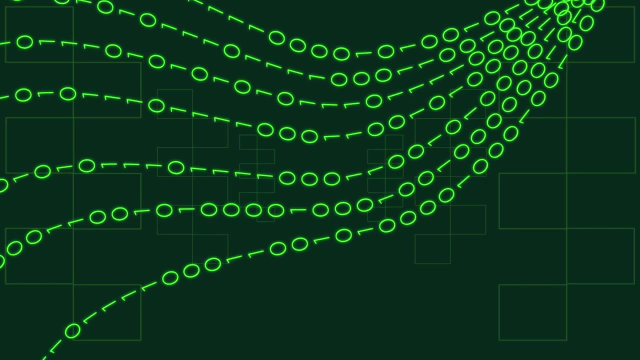 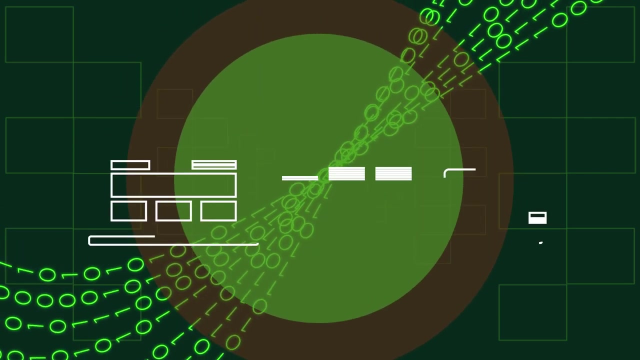 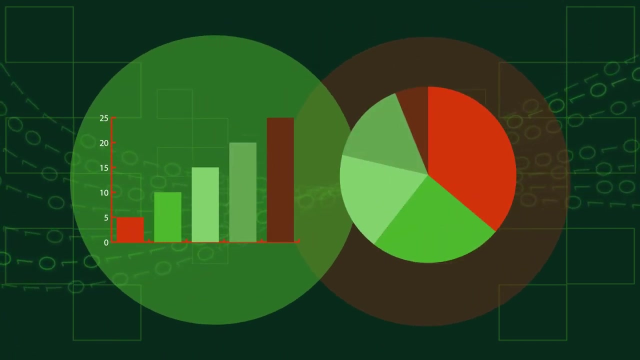 Data. Nowadays, information is being collected on everything. We have data coming out of our ears. These numbers might be showing us something very meaningful, but who can really tell? This is where bar graphs and pie charts come into play. They are really great for displaying data. 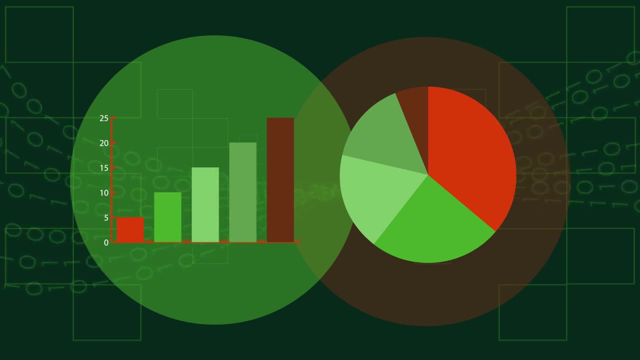 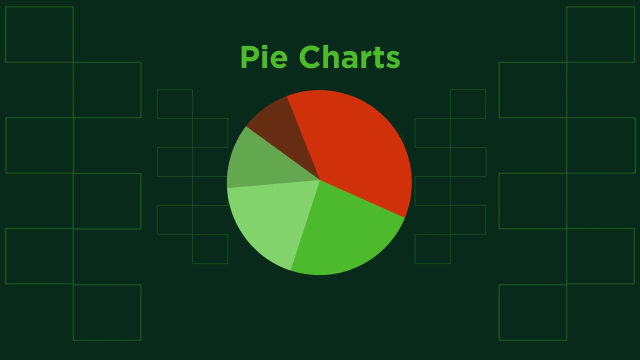 helping us to easily make comparisons on our data. In this video, we're going to look at pie charts in a little more detail. Sadly for pie charts, they come under fire from data experts who think they are inferior to bar graphs. They argue that pie charts are only suitable in rare circumstances. 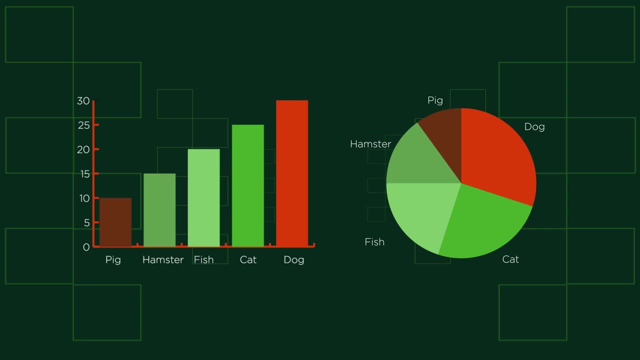 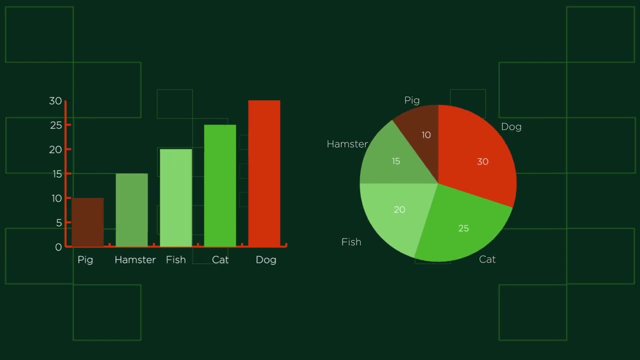 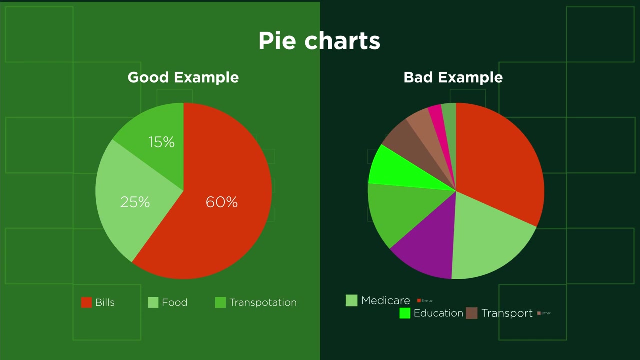 like here. We've used the same data set for both charts, but in the pie chart it's very hard to see any difference. Pie charts are only good for showing distributions if there are clear differences between each category. They should only really be used when there are less. 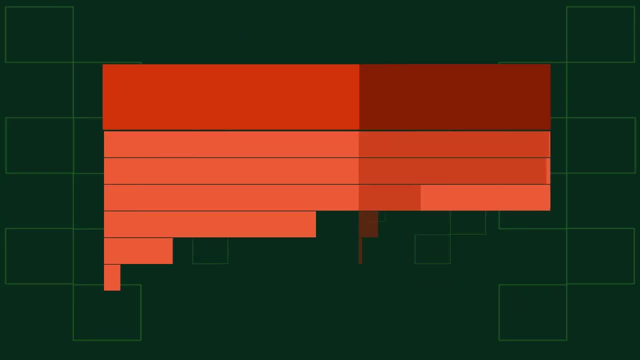 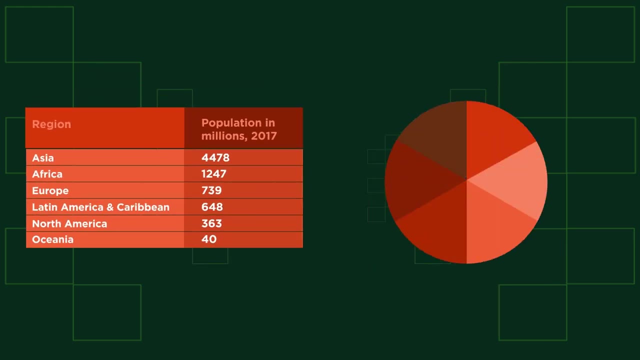 than six categories. So let's turn this population data into a pie chart. We need to work out what size each sector of the pie is going to be. You should already know that there are three hundred and fifty pie charts in the pie chart. We need to work out what size each sector of the pie is going to be. You should already know that there are three hundred and fifty pie charts. 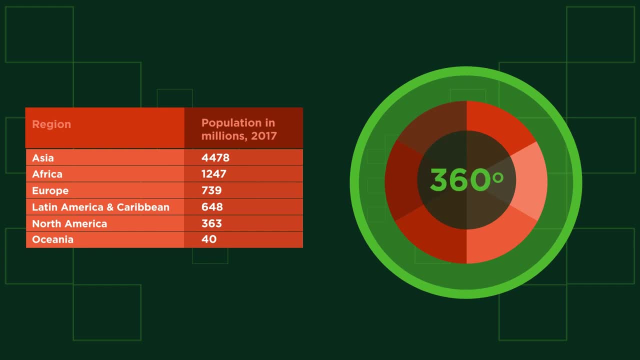 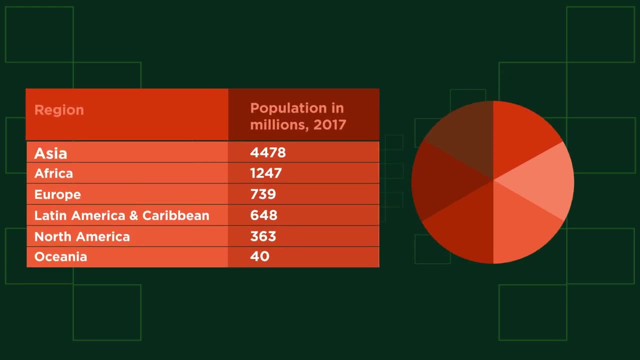 The pie chart is 360 degrees in a circle, so we need to share this 360 degrees out amongst our different categories. Asia has the biggest population, so needs the biggest slice. To work out exactly how big we need to add up all of the values. 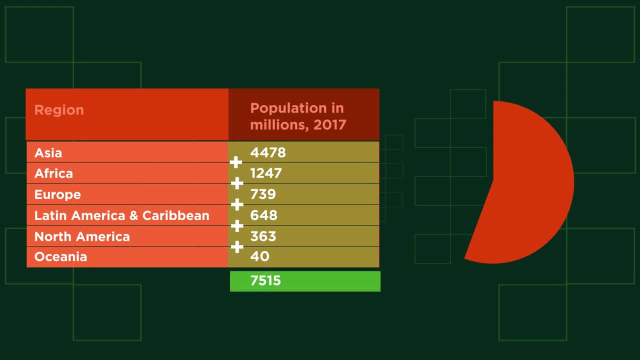 to work out the total population, which gives us 7515 million people in the world, which is actually seven and a half billion. The size of the Asia slice is four, four, seven, eight out of seven, five, one, five. 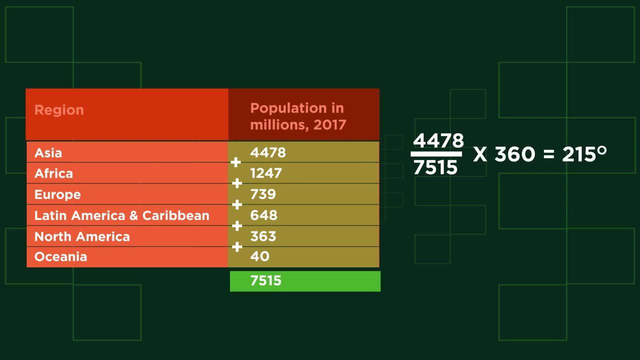 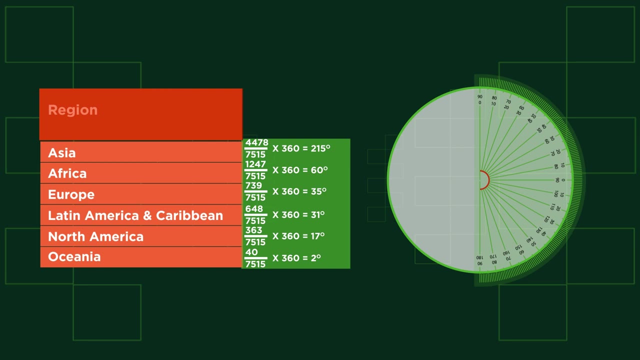 as a proportion of the full 360 degrees, Then Africa, Europe and the rest. With your protractor, you can now divide your pie chart up by these degrees, Starting from the vertical measure, 215 degrees clockwise, and label this sector Asia. 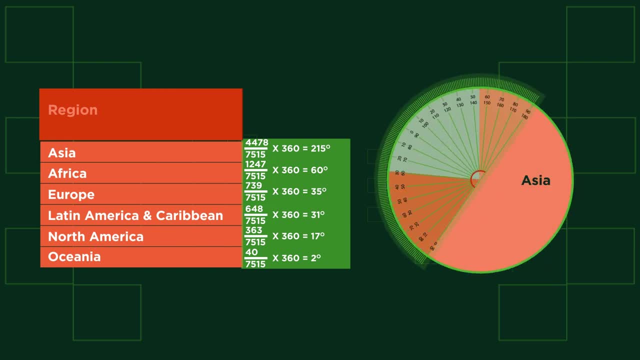 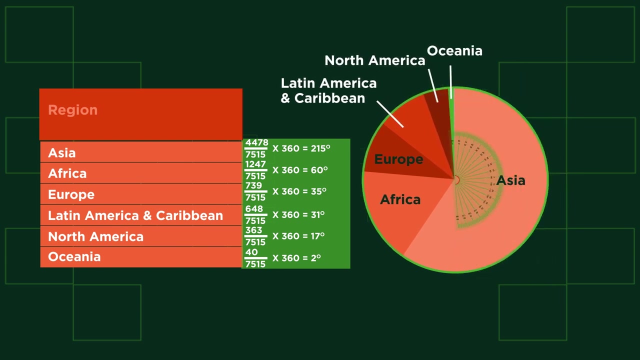 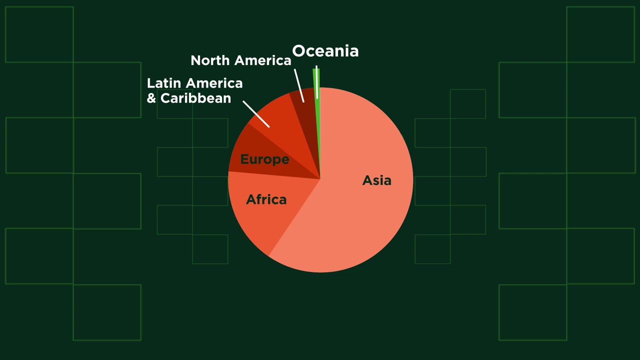 Then measure 60 degrees and label it Africa, 35 degrees for Europe and then, finishing off, the last three. This works as a pie chart. Asia is clearly the biggest, getting smaller until Oceania. Good pie chart practice is to start with the biggest sector. 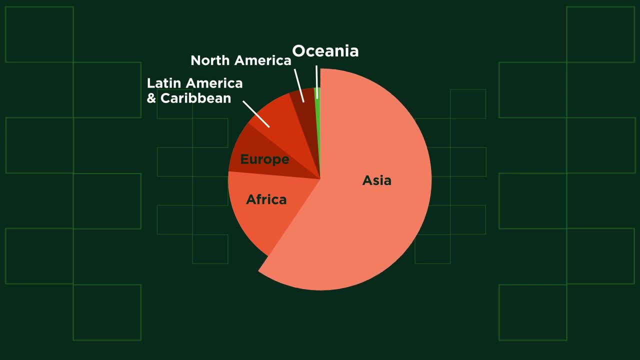 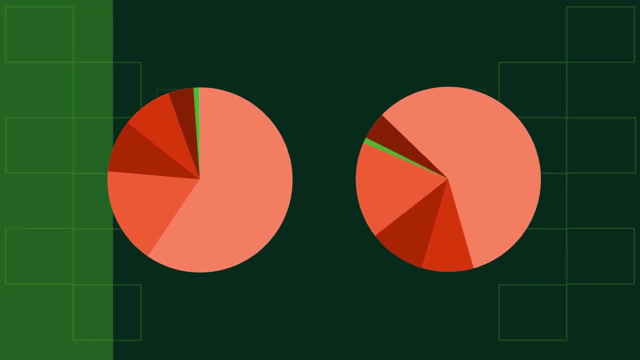 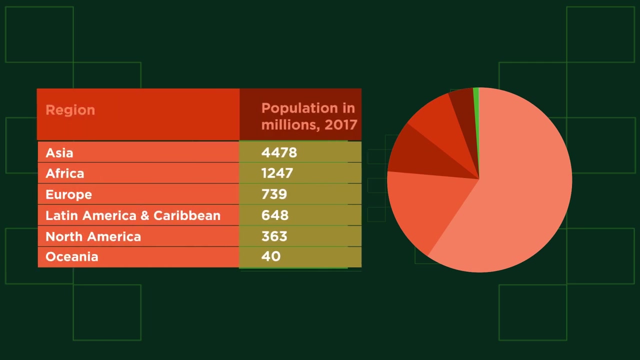 so Asia, and then work your way clockwise, doing the next biggest Africa, then the next biggest Europe, and keep going in order of size. It massively helps the viewer. Pie charts often also have the percentage written on them. What percent of the world population? 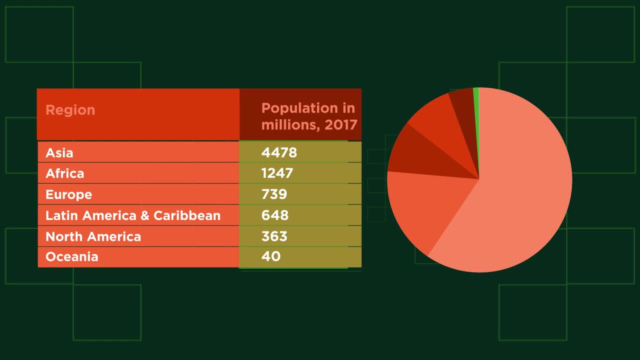 does each region contribute? So we go back and turn the populations out of the total world population into a percentage. Nearly 60% of all people live in Asia. Can you work out what percentage of people live in each of the other regions? Pause the video. find the percentage. 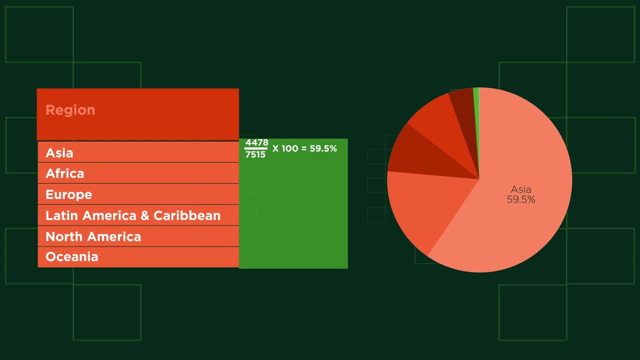 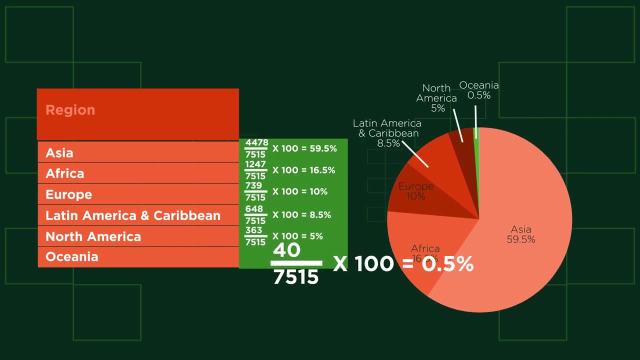 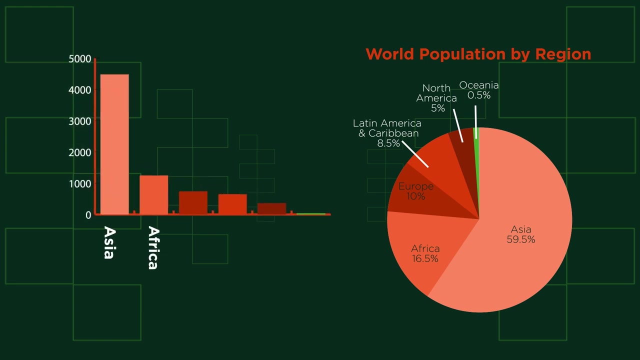 and click play when you're ready. Did you get them right? And, as with any chart or graph, we need a title. A bar chart would have done just as good of a job. but A bar chart would have done just as good of a job. but. 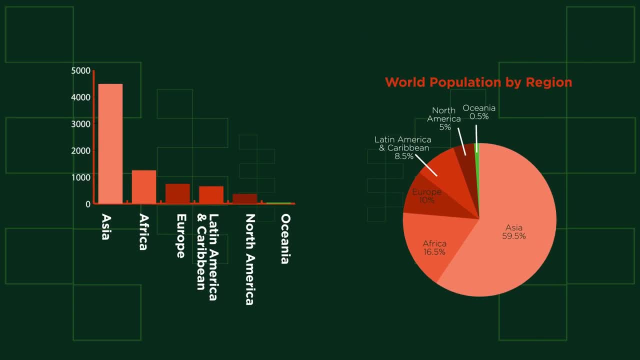 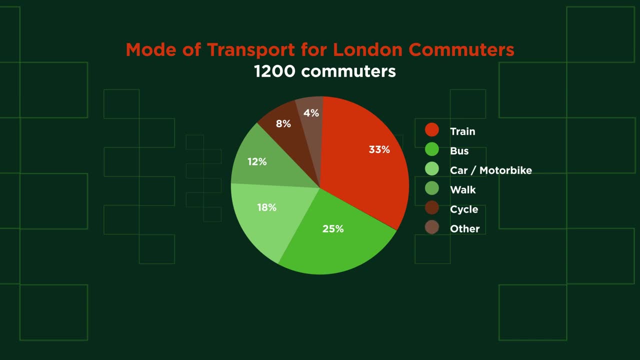 a pie chart hasn't done too badly here. Sometimes questions might give us a pie chart with a percentage already on and then they ask us to find what this represents. So we know that 25% of the 1,200 travelled by bus.